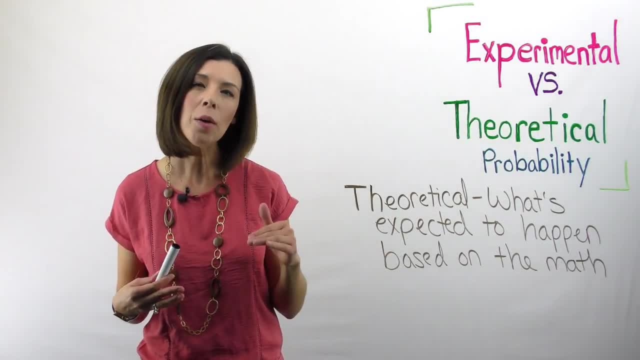 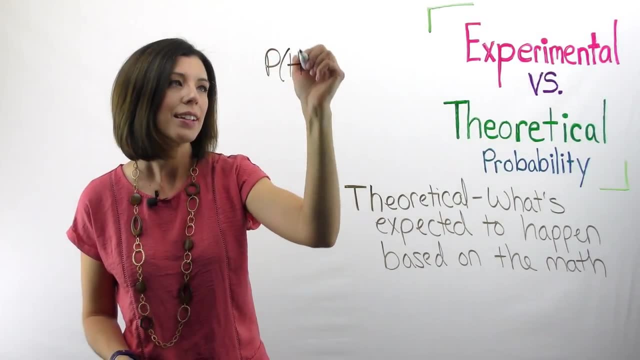 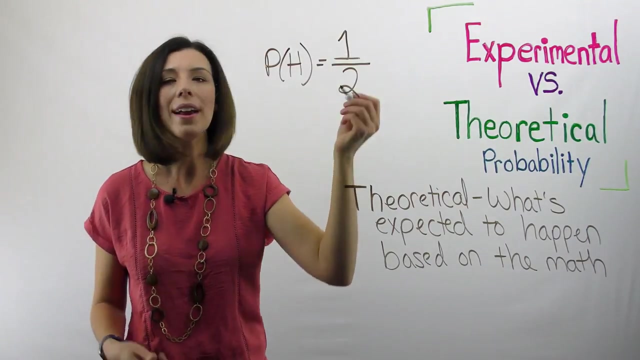 that are possible outcomes in the situation, and then how many of those outcomes would give me the desired event. If I'm finding the probability of heads, I know that there are two possible sides on a coin- heads and tails- and I know that there is just one head. My theoretical probability is: 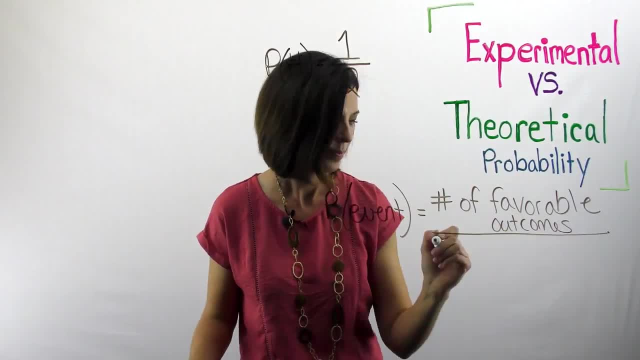 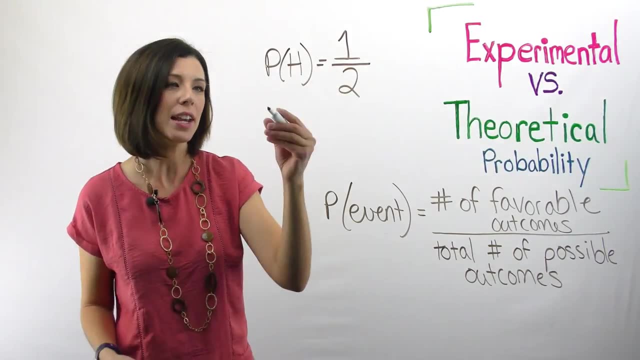 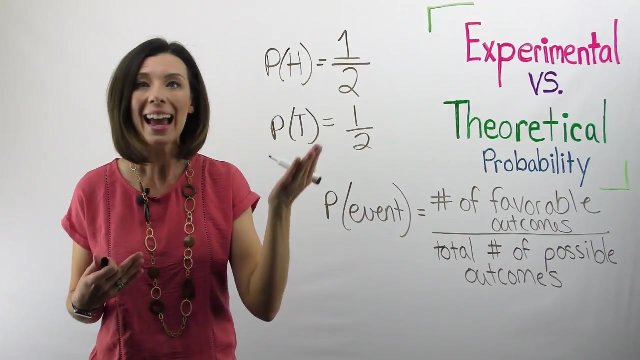 one half, Just like I can find the probability of heads- that's one half- and also find the probability of tails, which in this case would be the exact same thing. right Again, I still have two options: Favorable outcomes or tails would be one out of two. 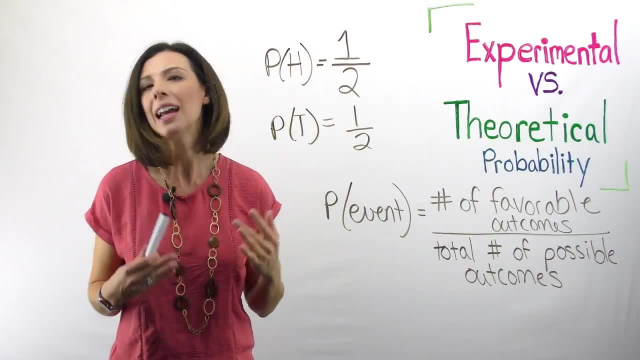 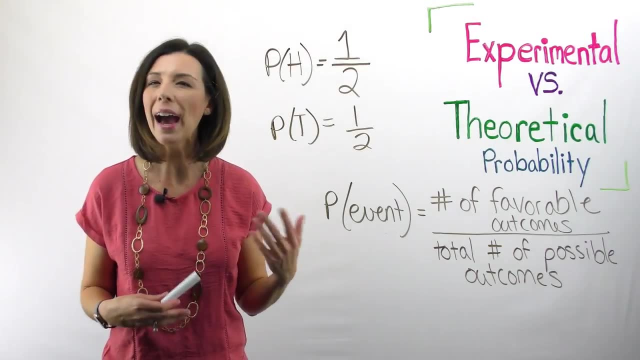 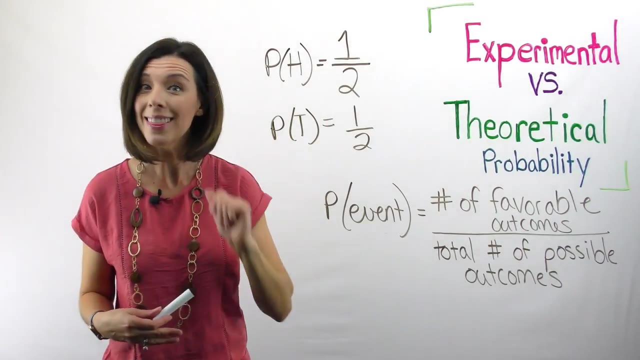 possibilities. This would be theoretical probability. Here's where it gets tricky and where we start to distinguish the two. Experimental probability is when you actually start flipping the coin. In theory, we should be able to get heads one out of every two flips. in theory, 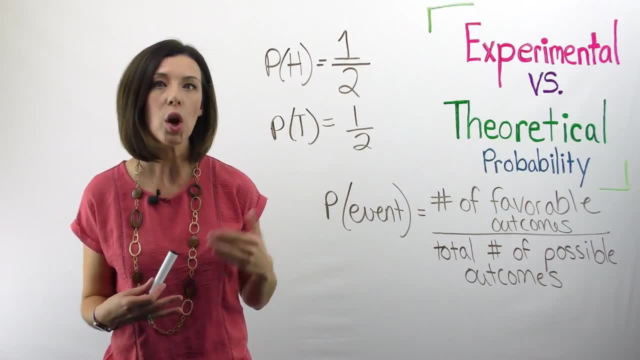 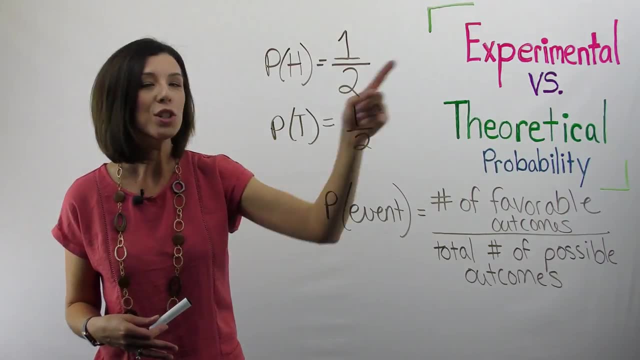 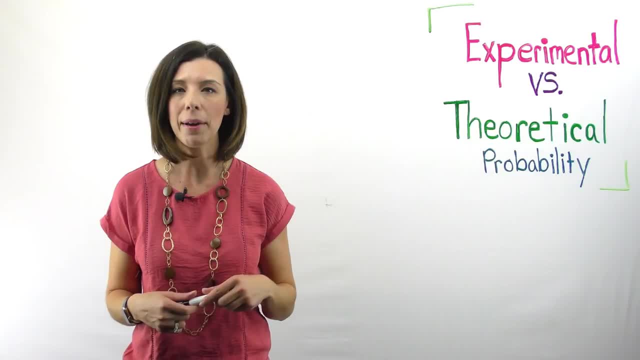 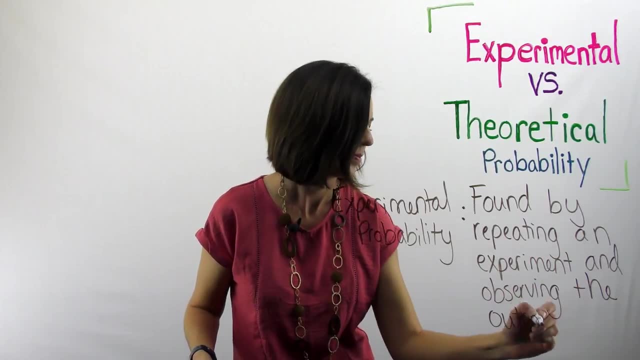 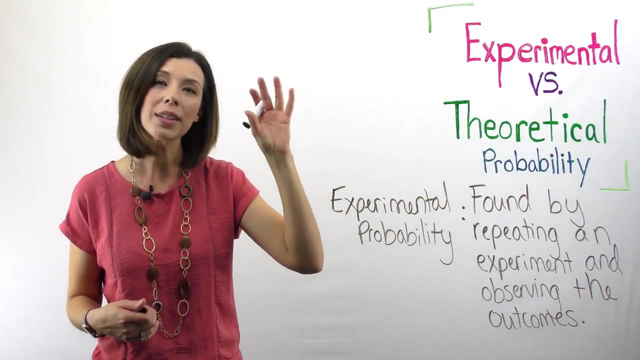 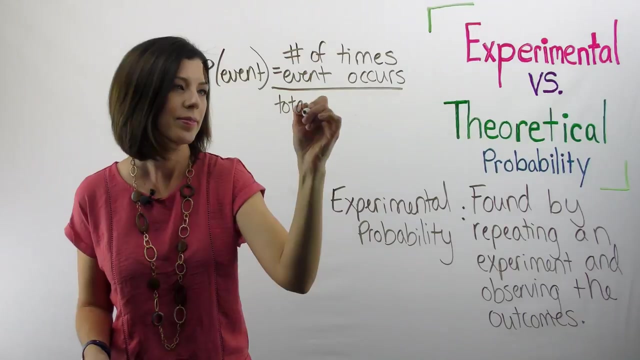 the outcomes. We have a different equation for how we want to think about this. For experimental probability, we want to write our fraction as the number of times the event occurs out of the total number of trials. Let's go back to our flipped coin and look at this through the experimental probability lens. 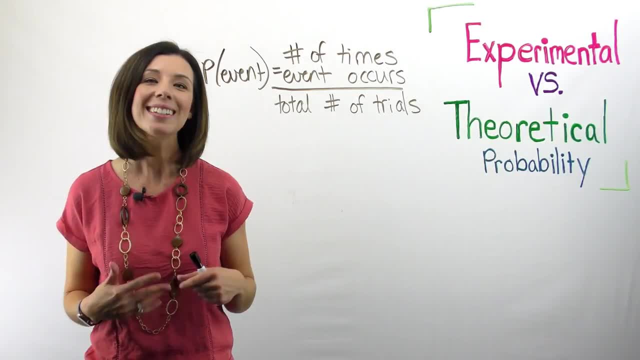 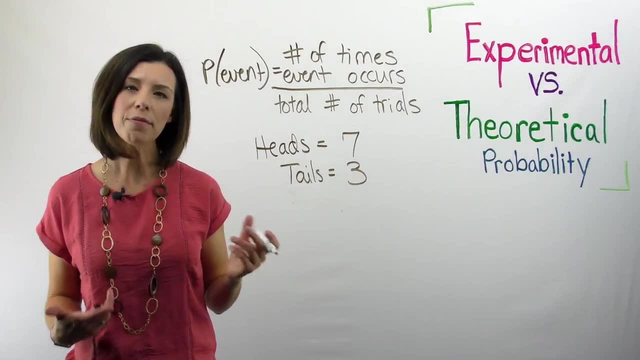 Let's say that I flip a normal two-sided coin. Let's say that I flip a coin 10 times in a row. Let's say that three of those times I get tails and seven times I get heads. If I'm thinking about what's the probability for getting, let's say: 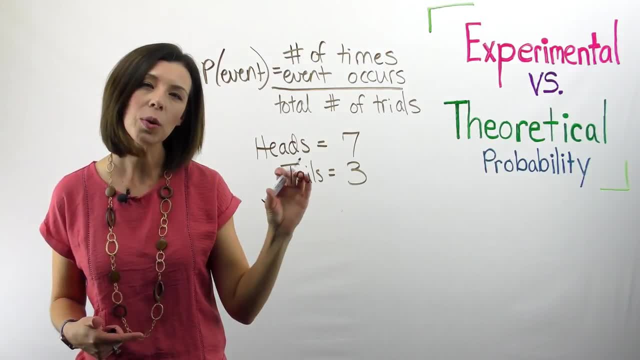 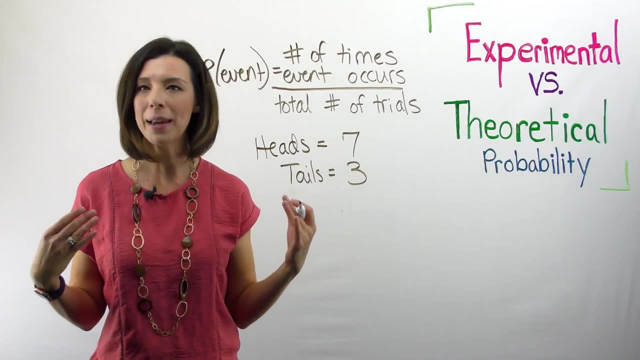 heads. I'm going to think about that. I flipped the coin 10 times and I got it seven out of 10 times. Now, remember this is what actually happened to me. This is not based on the math. Based on the math, I had my probability of one half right. This is based on what actually